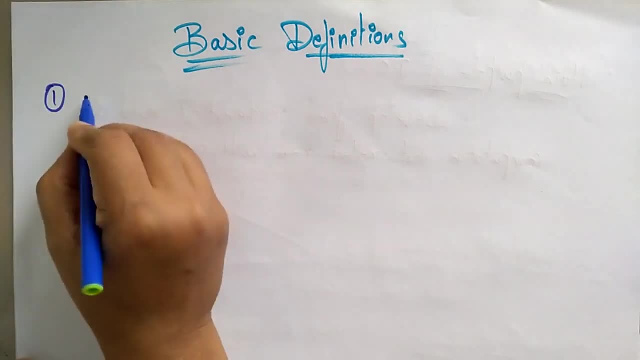 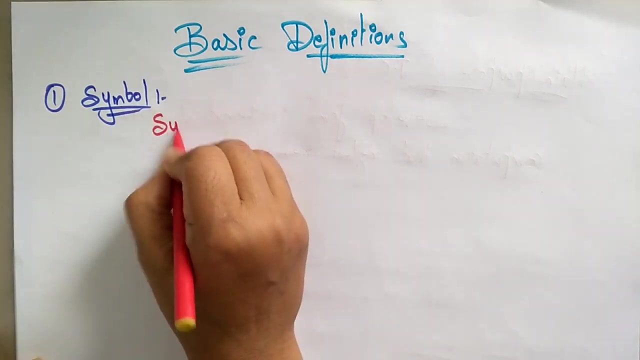 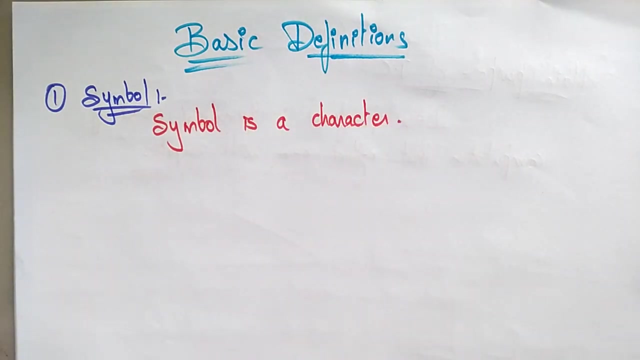 Okay. so first thing is the basic definition that you have to know is symbol. So we use the term symbol and this theory of computation. So what this symbol indicates? A symbol here is nothing, but it is a character. Symbol is a character. Okay, so what is this? characters, Characters are. 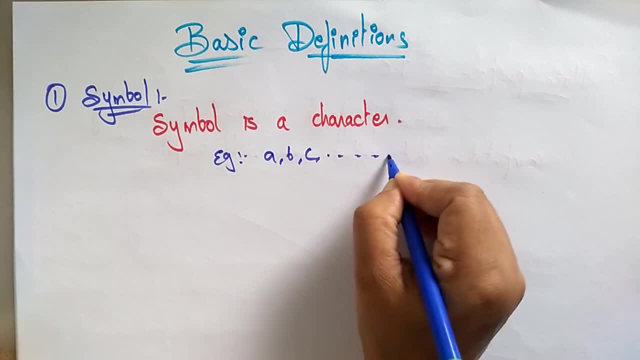 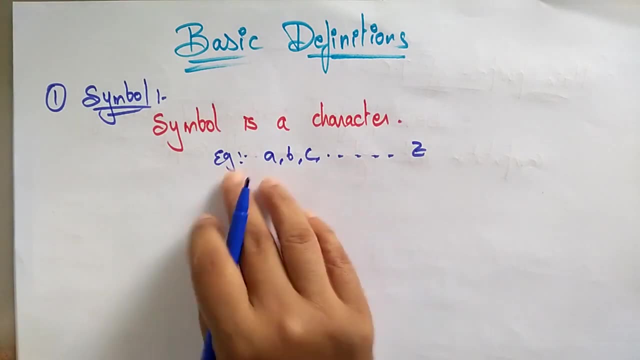 nothing but example: A, B, C, up to Z. So each letter, you call it as a symbol, Each character, you call it as a symbol. or even not only that, Alphabets, the numbers, also numeric values. up to 9 is also a symbol, 0 is a symbol, 2 is a symbol. 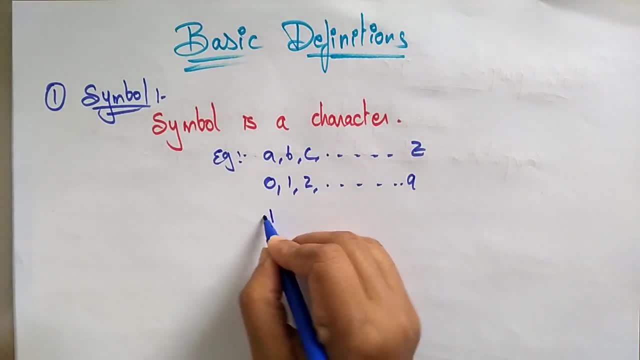 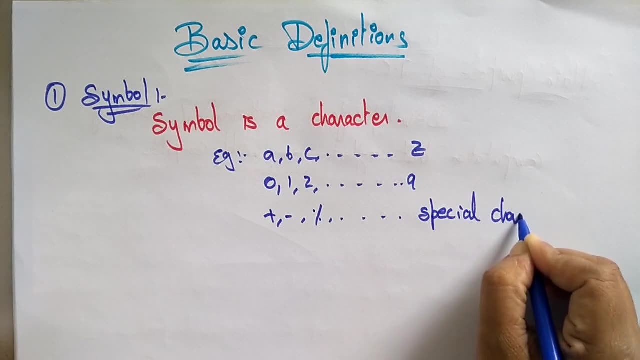 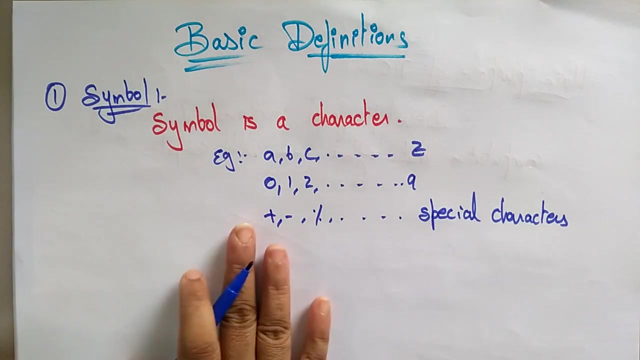 8 is a symbol, 7 is a symbol, and even the special characters like plus, minus, modulo. Okay, you call it as a special characters. These are also. you call it as a symbols. So whenever you have seen a letter, a character or a number or a special character, then you call it as a symbol. 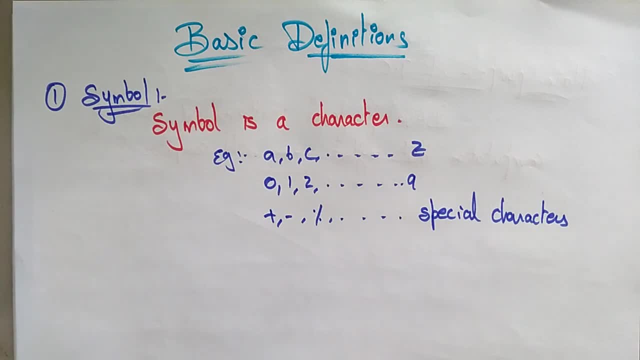 not an alphabet, Not a number. Okay, so in the theory of computation you call: symbol is a character. So whenever you have seen the character, you have to call it as a symbol. Now coming to the next definition. Next is alphabet. So you will get a doubt Here. these are the alphabets. Again, what is? 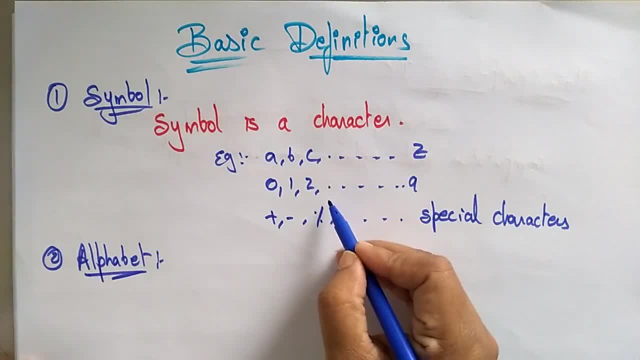 this alphabet. I am saying here the alphabet is a symbol, Okay, but I am taking another definition: alphabet. Okay. So there is no confusion: A set of characters. you call it as an alphabet. Set of characters, not a single one. Set of. 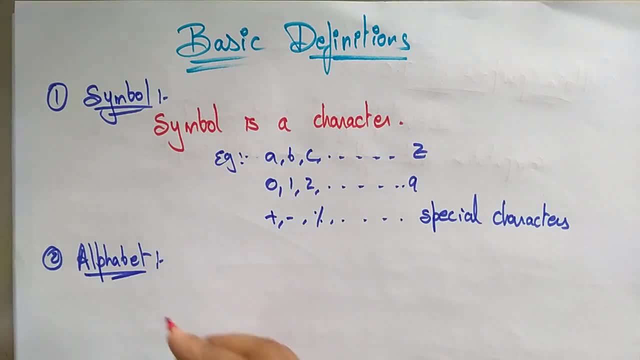 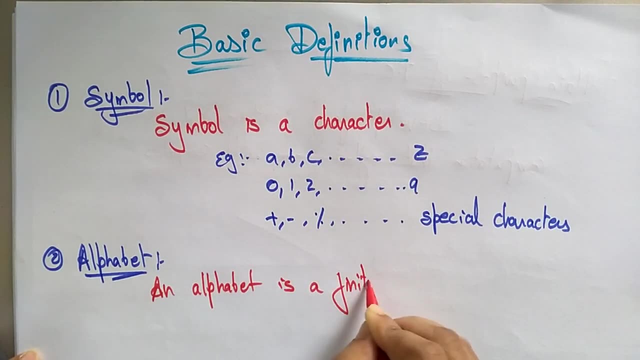 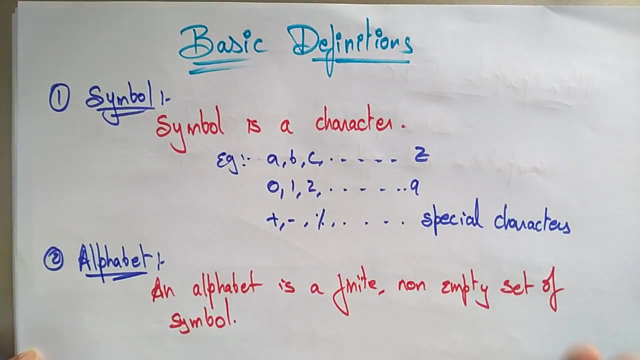 characters. you call it as an alphabet. Okay, let me write: An alphabet is a finite. non-empty set. Remember that Means something has to be there. It should not be non-empty set Of non-empty set of symbol. A non-empty set of a symbol. you call it as a finite. It is a. you call it as an alphabet. 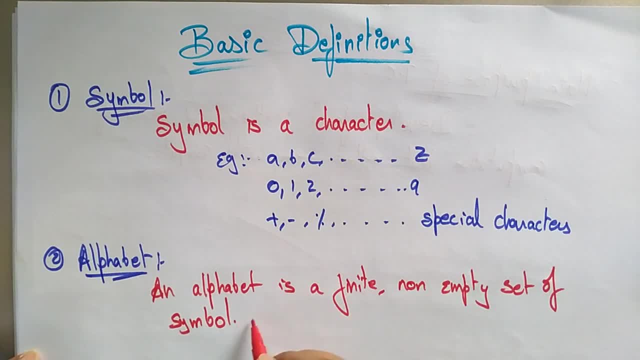 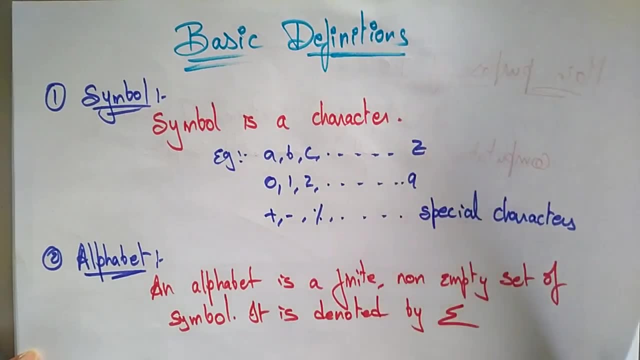 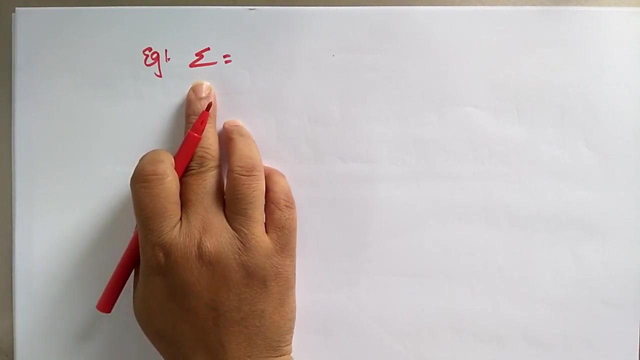 So an alphabet is a finite, non-empty set of a symbol and it is denoted by and it is denoted by sigma. It is denoted by sigma. Let me take the example. Suppose sigma. Whenever you have seen the sigma in this theory of computation, you have to call it as an alphabet. Okay, 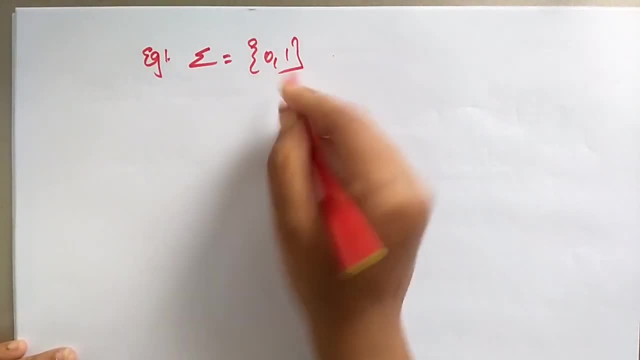 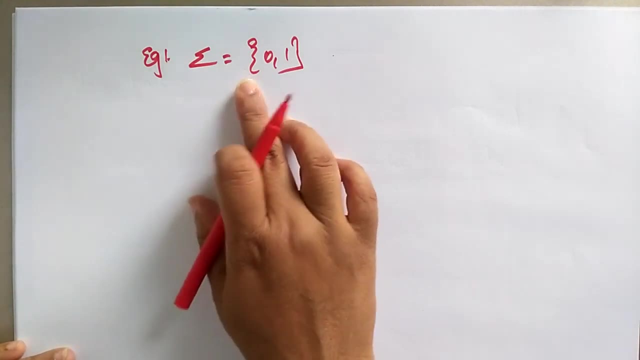 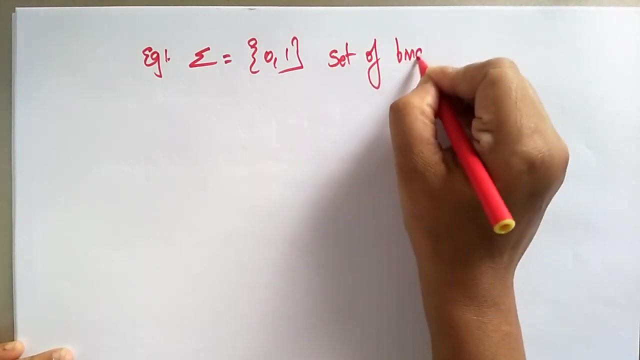 A sigma is set of finite, non-empty set, 0, 1.. It is a set. The set can be represented with open parentheses and the closed brackets. Okay, So this is set of. you call it as a binary alphabets. So what are the binary alphabets? The binary alphabets are nothing but 1 and 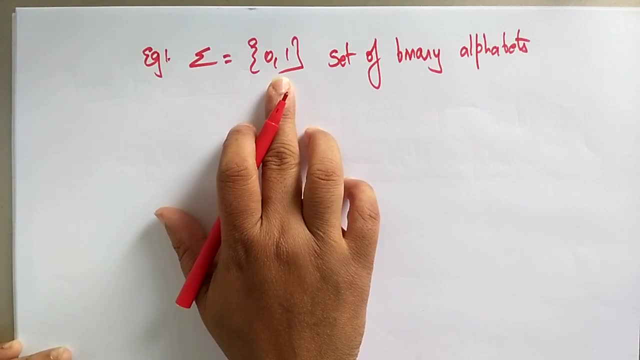 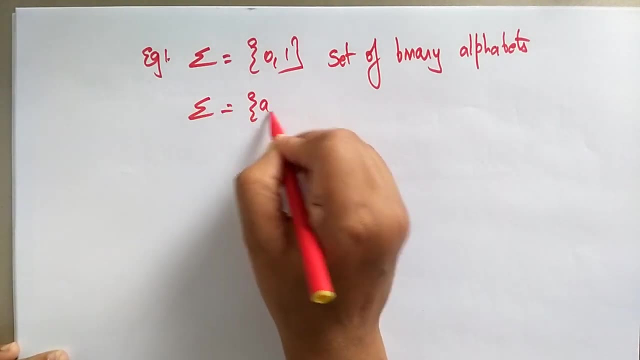 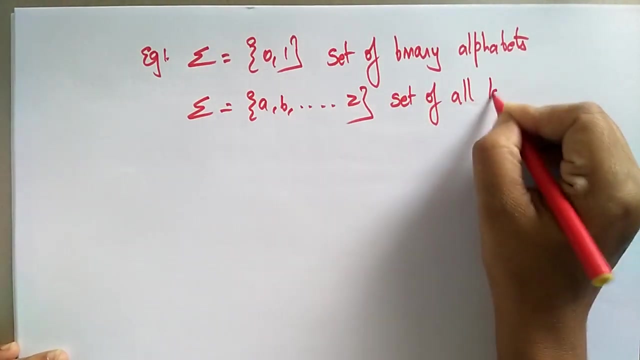 0s are the binary numbers, So if it is set a set of binary alphabets, you call it as an alphabet. Okay, And sigma is equal to. let's take a, b up to z. This is set of all lower case. 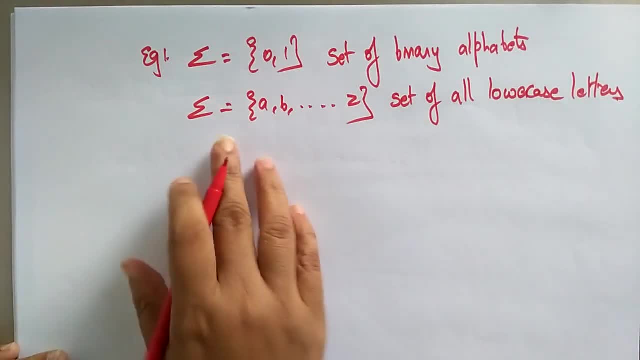 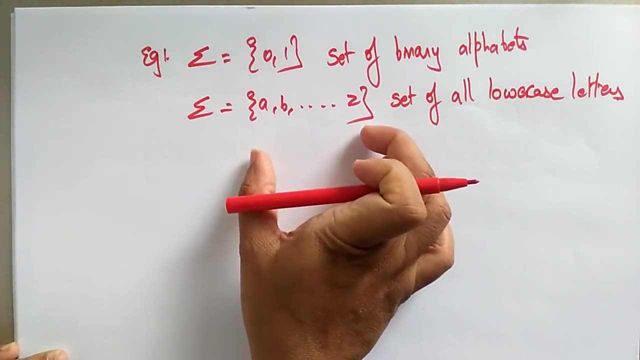 letters. So you have to remember that the alphabet is denoted with sigma. Whenever the sigma is there, a set should be there A set it should be. a non-empty set Means you have to include any single character in the set. 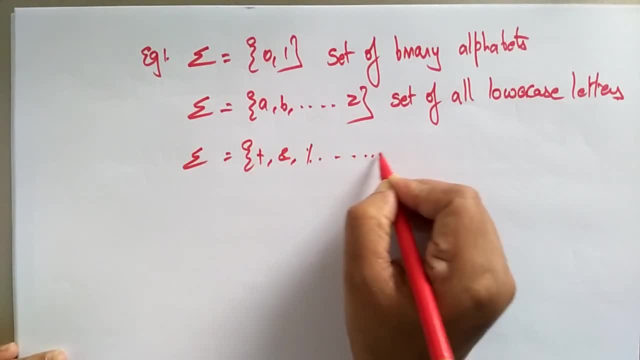 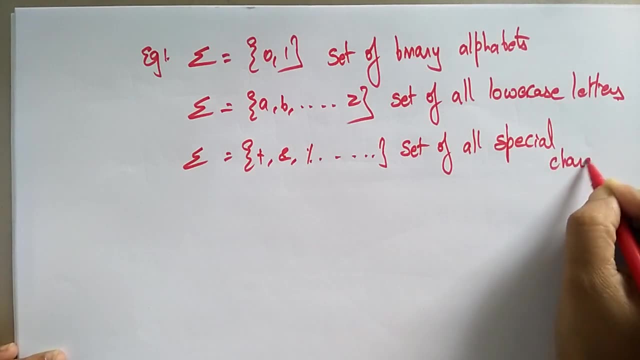 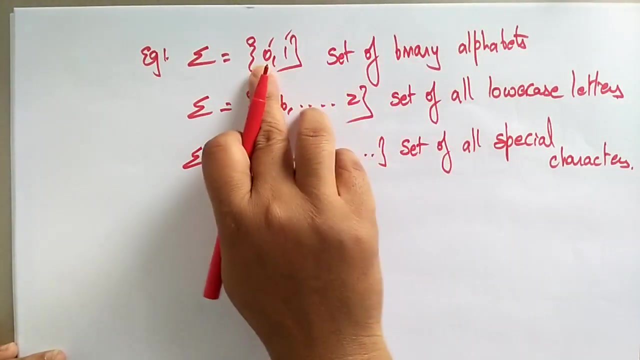 Example. let me take the special characters also. These are all the set of all special characters, Special characters. So I hope you understand what is the definition of the alphabet. So the basic definition here: each character, you call it as a symbol and the 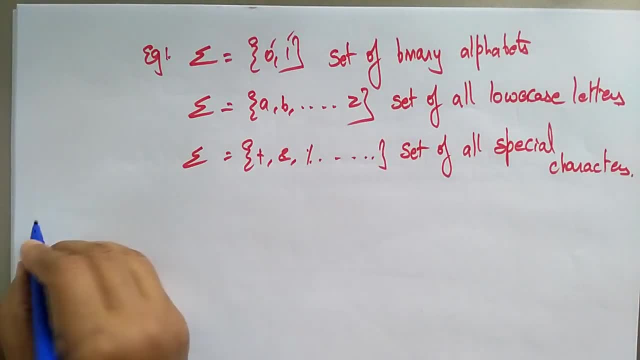 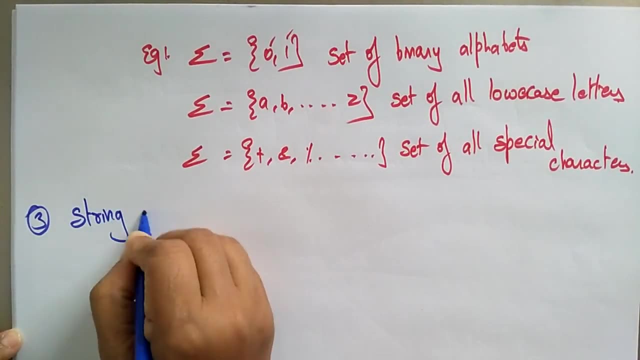 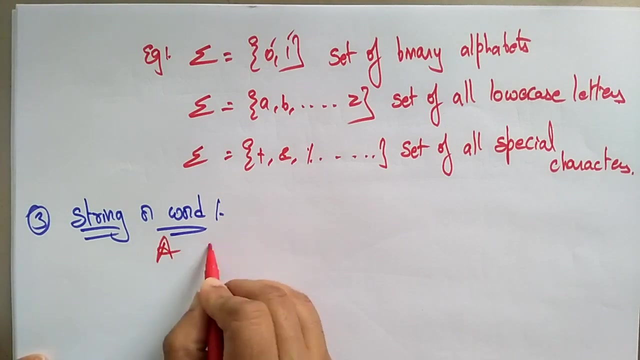 set of those symbols. you call it as an alphabet. And next definition, come to the next definition. There is a string or a word. Even you call it as a string, Or simply you can call it as a word. also, A string is a finite. A string is a finite. 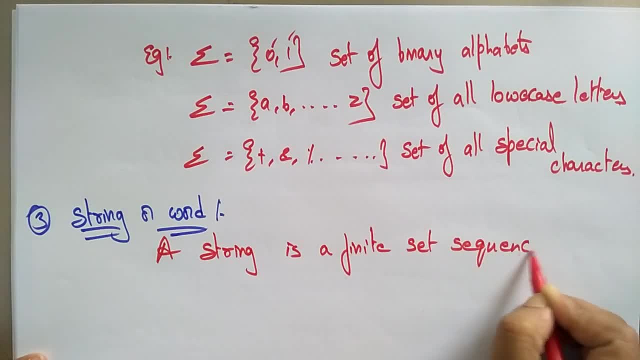 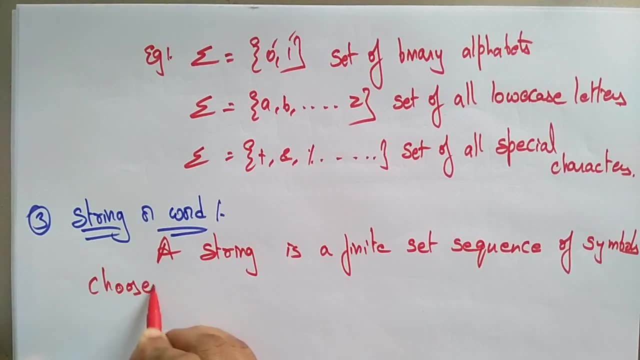 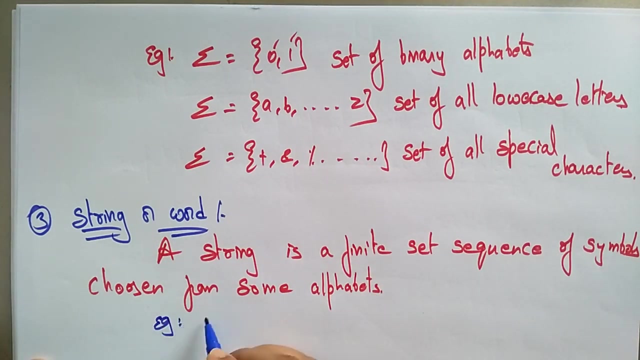 Set sequence of symbols. Set sequence of symbols. Remember this: A sequence of symbols Chosen from some alphabets, From some alphabets, means either you can chosen from this, or you can chosen from this, or chosen from this some alphabet. let me take example here. let me take the example. let's take a set of a string. 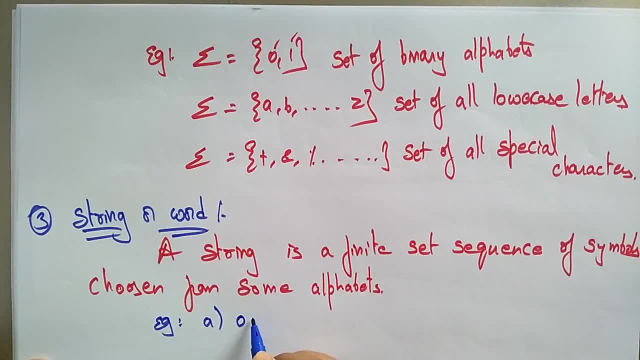 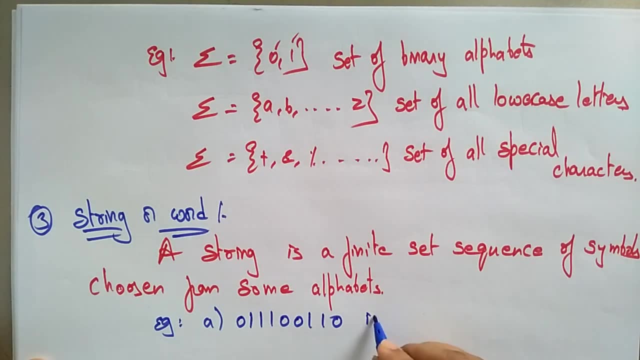 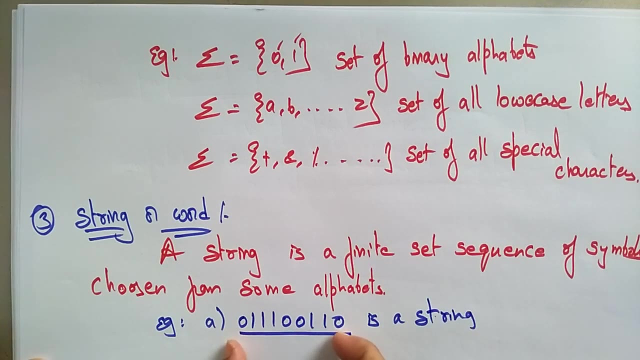 is a finite sequence of symbols. here i am taking a sequence of symbols like: zero is a symbol, one is a symbol, one is a symbol: zero, zero. so so what do you call this? so it is a string. you call this complete as a string, or you can call it as a word string or a word from. 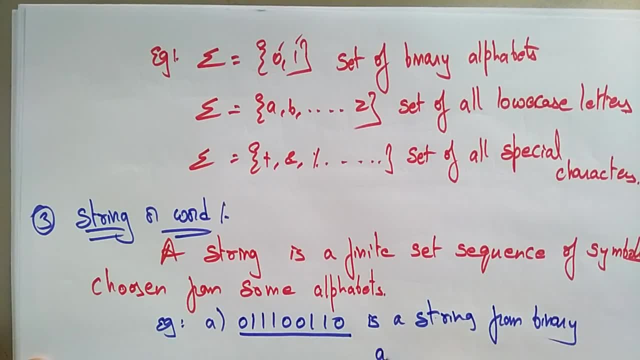 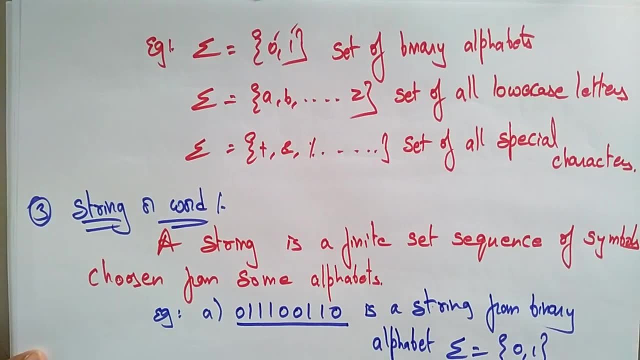 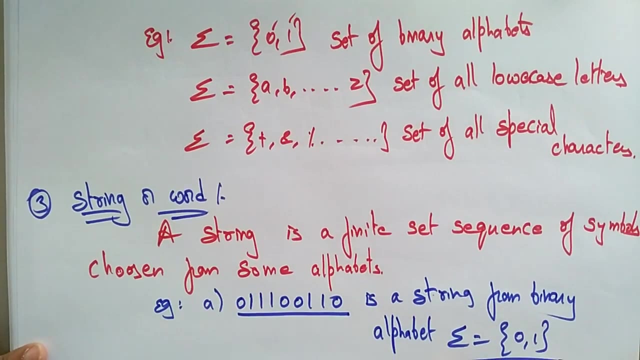 binary alphabet of set sigma is equal to zero comma one, right, is it correct? i have taken this. i have implemented this word or a string by taking the alphabet of set zero comma one. so a string is a finite set sequence of symbols chosen from alphabets. 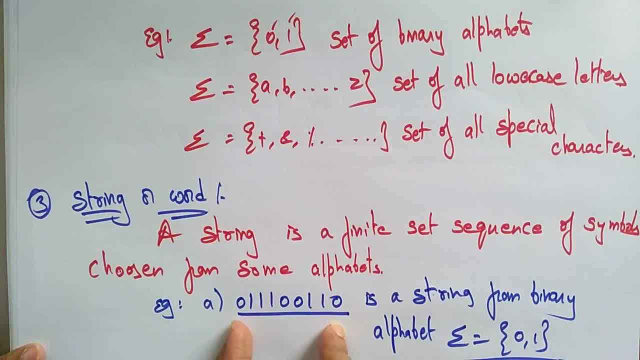 i have to chosen from these alphabets. that is a, c. i have chosen this word from these alphabets, that is 0 comma 1. i have written like 0, 1, 1, 1, 0, 0, 1, 1, 0, like this: okay, let me take another example. so, 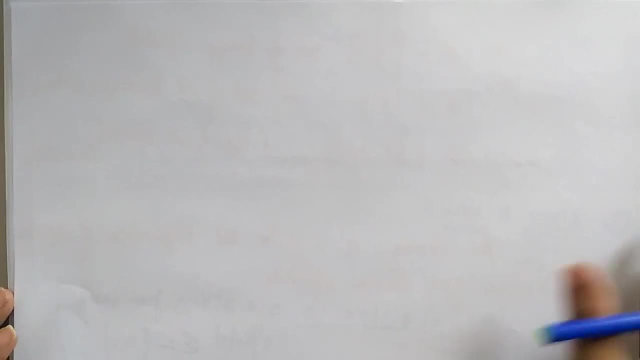 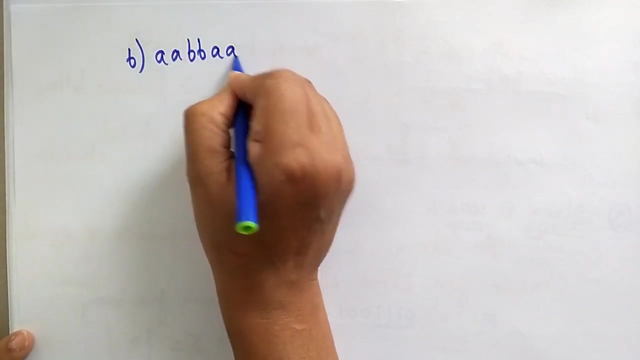 that we understand what exactly the string or a word is, and i am saying it is taken from the set of alphabets. let me take a, a, b, b, a a, c, a b, so i call it as a string. it is a string or you can. 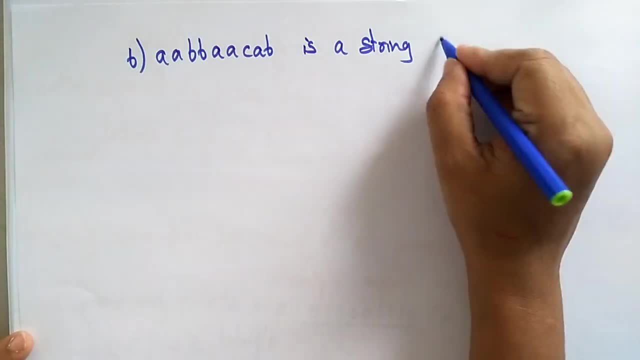 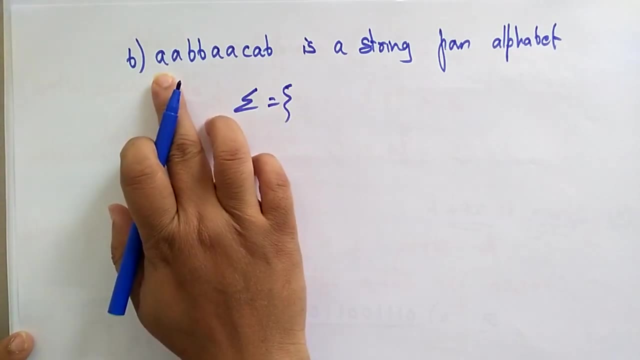 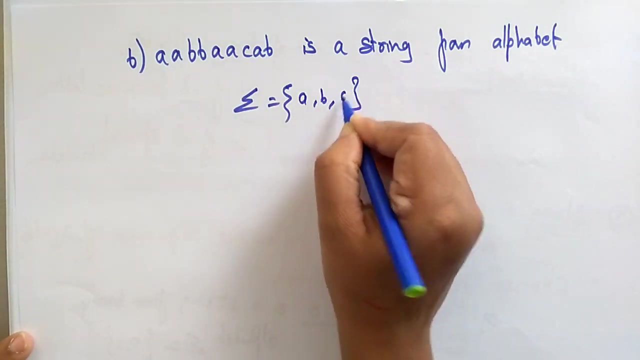 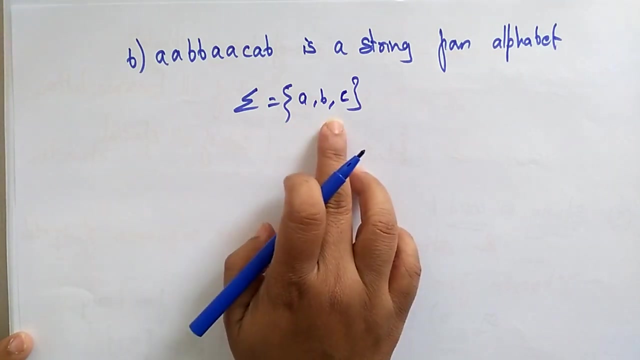 call it as a word. so i have taken this string from alphabet, alphabet set, what i have taken. so here: a is there, b is there, c is there? only three letters are there. so i have taken from this three letters. a string from the alphabet of set. sigma is equal to a, comma b, comma c. 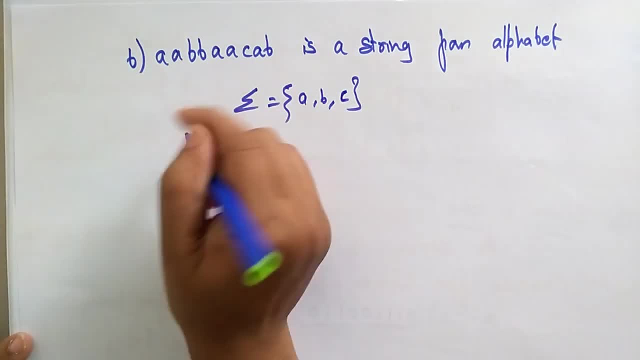 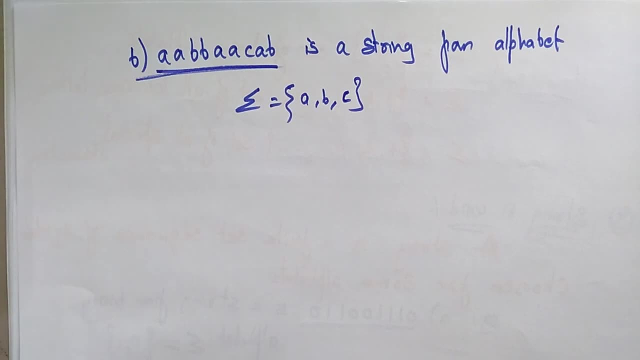 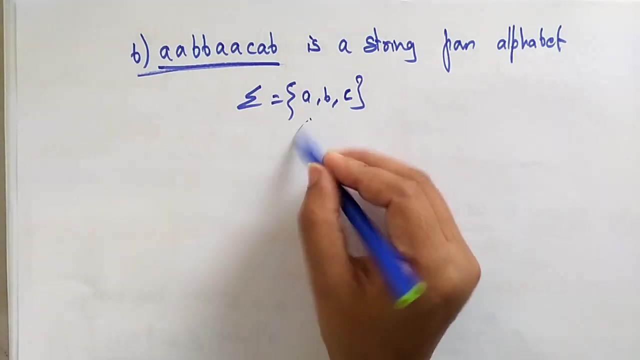 so from these three letters, characters, i have implemented this word. so that is a string, a string or a word, you call it as it is, a finite set, sequence of symbols chosen from some alphabet, some alphabet, so don't confuse. each letter in this alphabet is a character, or you call it as a symbol and set of that symbols, you call it as an. 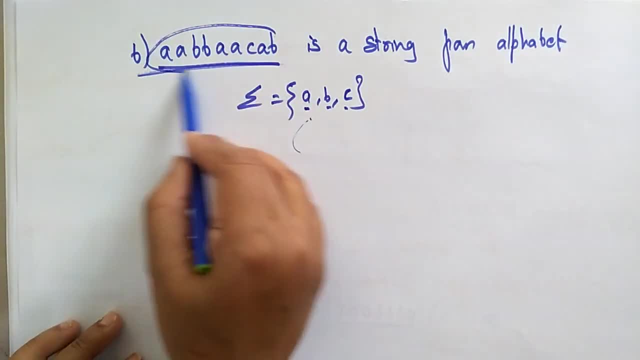 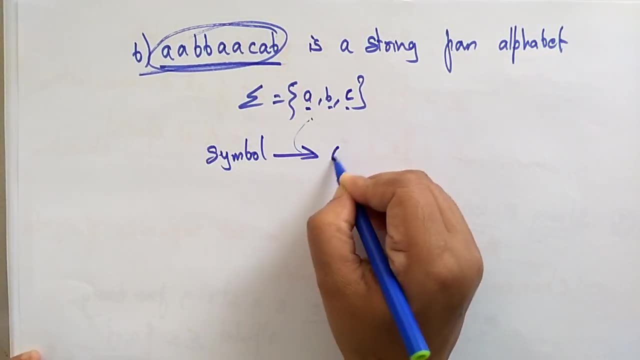 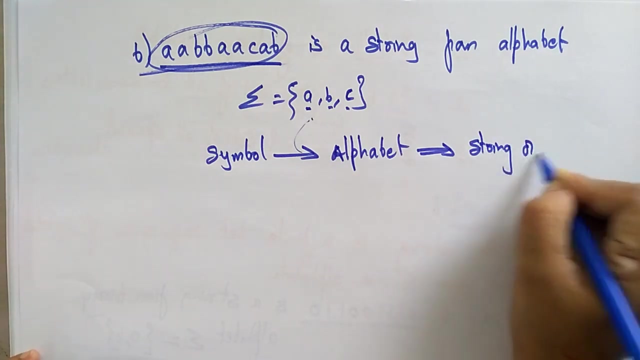 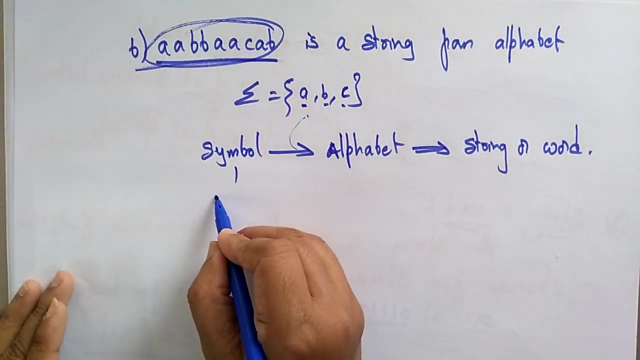 alphabet. in this alphabet we are developing a string or a word. okay, first symbol, symbol to alphabet from the set of alphabets, we are writing a string or word. so i hope you understand what exactly the symbol is: a symbols or nothing, but the letters a or one or zero, like.